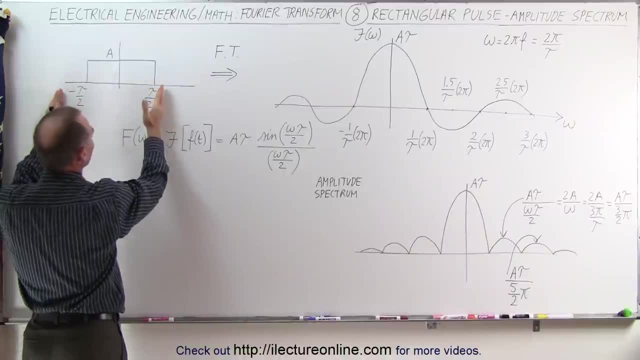 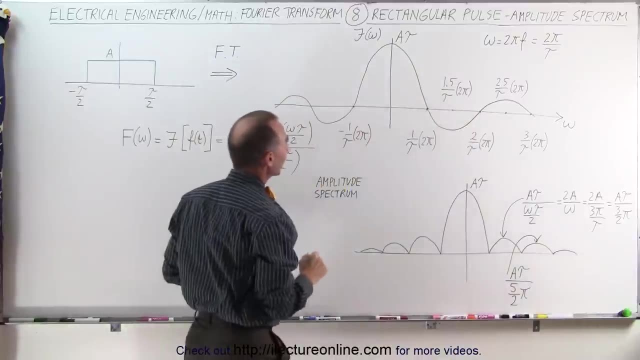 So it starts from minus tau over 2 to tau over 2.. And if we take the Fourier transform of that we get this function right here. It looks kind of like a Bessel function. It has an initial amplitude of A times tau. 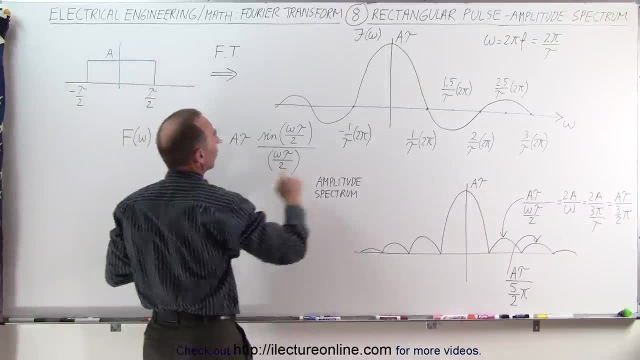 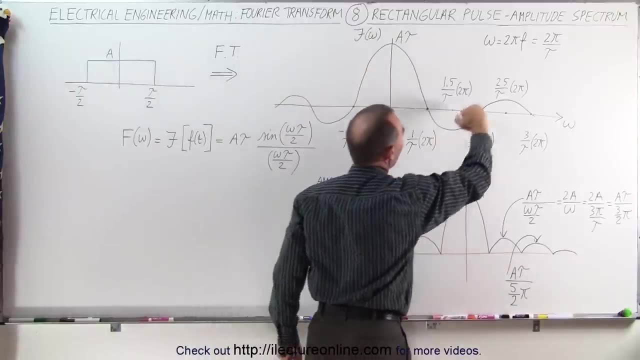 A is the amplitude of the pulse and tau is the pulse width. So the amplitude here would simply be the product of the amplitude here times the pulse width, And then you can see how the amplitude tends to oscillate and become smaller and smaller and smaller. 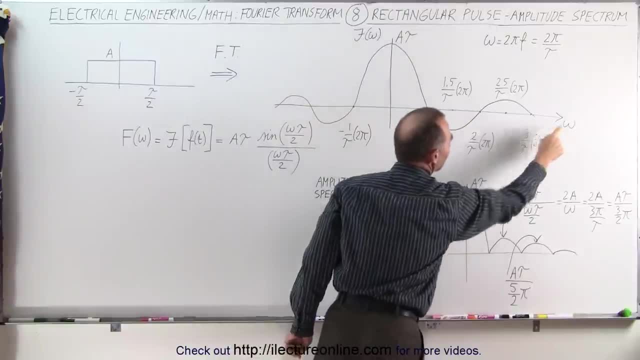 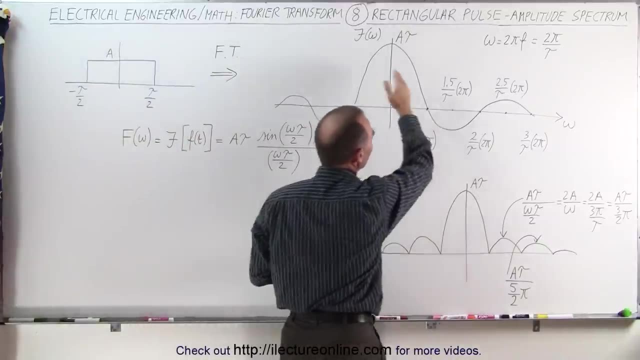 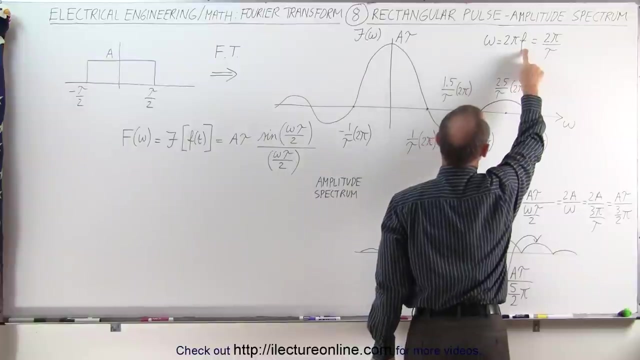 The question is, where does it cross The frequency, The frequency axis? And so what we're doing here is we go from the time domain to the frequency domain, And we're trying to understand this curve a little bit better. Notice that the angular frequency is equal to 2 pi f. 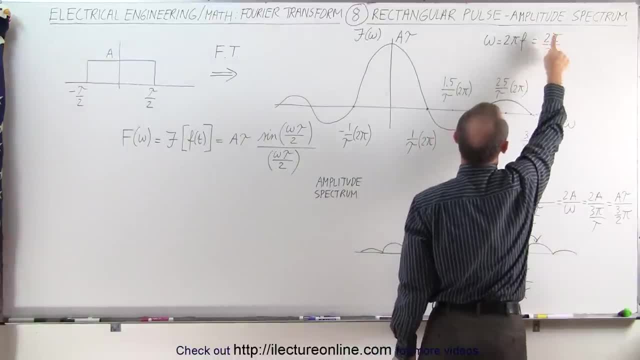 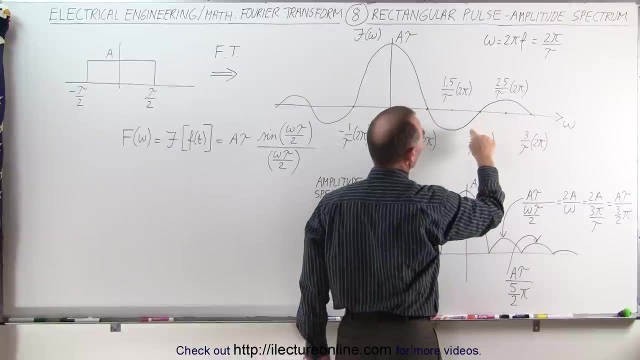 And f is 1 over the period. So omega becomes 2 pi over the period. Notice that it crosses over here at 2 pi over the period. Then here it crosses over at 2 times 2 pi over the period And it crosses again at 3 times 2 pi over the period. 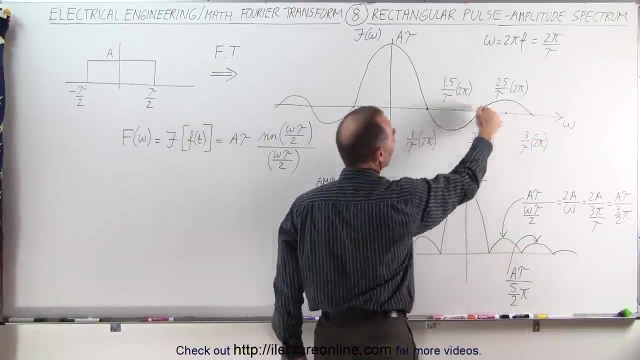 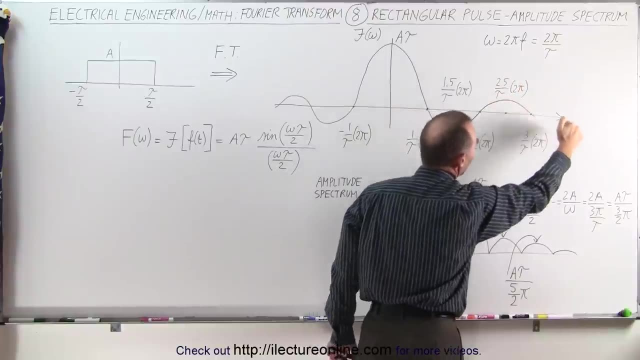 And so forth, The points in between where you have an amplitude. Here we have 1 and a half times 2 pi over the period, And 2 and a half times 2 pi over the period, And 3 and a half and so forth. 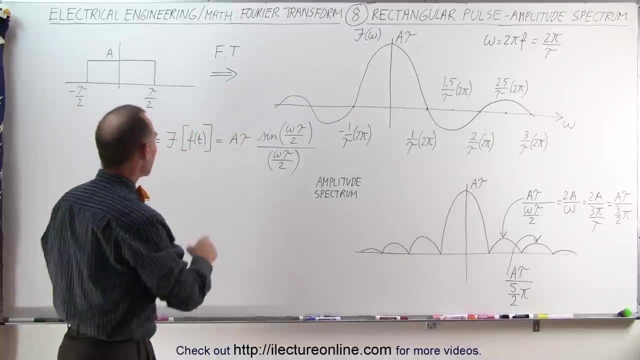 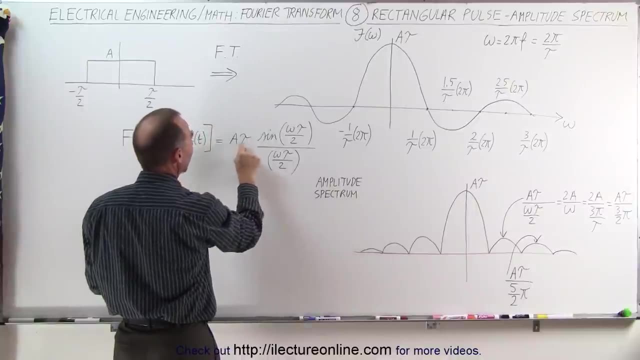 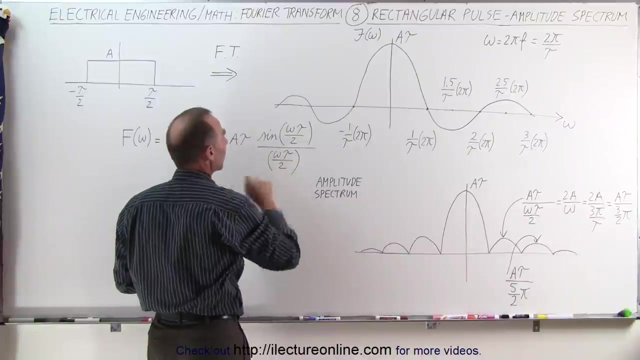 So you can see the pattern Here. we notice that the amplitude of that function can be described by the product A times tau, which is this amplitude right there, Times the sine of omega tau over 2, divided by omega tau over 2.. Now that's the function that describes what you see over here. 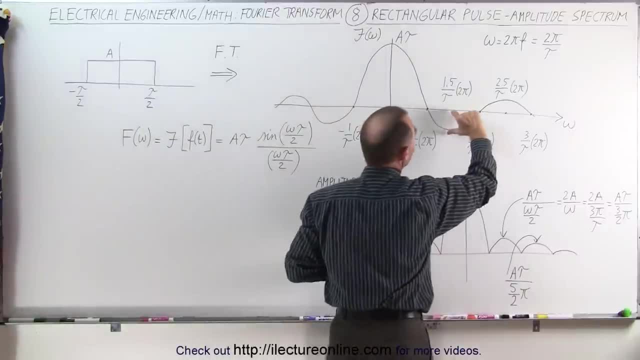 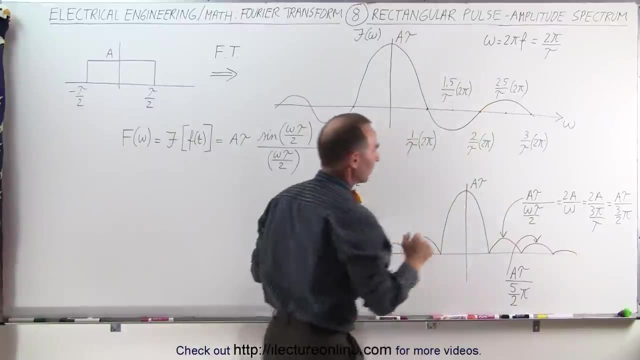 If you don't want to have the amplitude, you simply take every negative portion of the function and flip it over and make it positive. So that would simply be the amplitude spectrum of what we see over here. Again, the amplitude of the middle is just like it's over there. 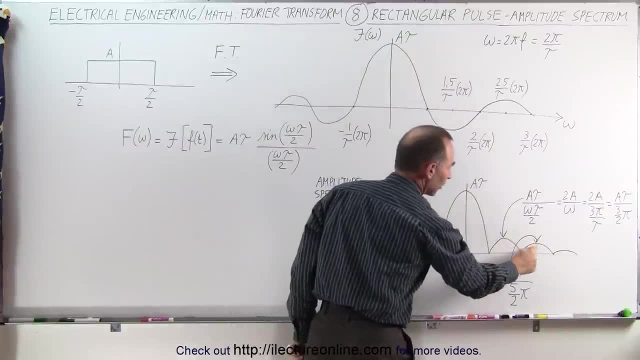 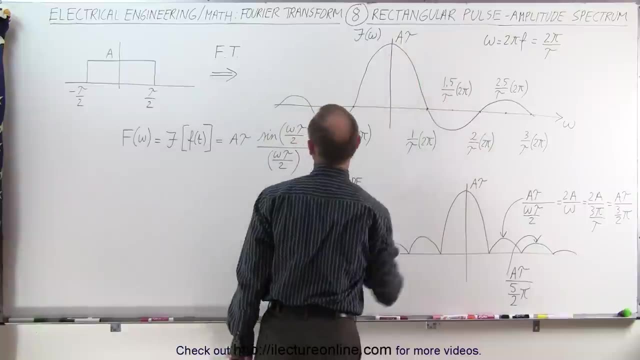 A times tau. So what is the amplitude there, there and there and so forth? And we'll get to that in just a moment. First of all, the amplitude over here. Why is it A times tau? Well, if this is the function, notice the sine of an angle divided by the angle. 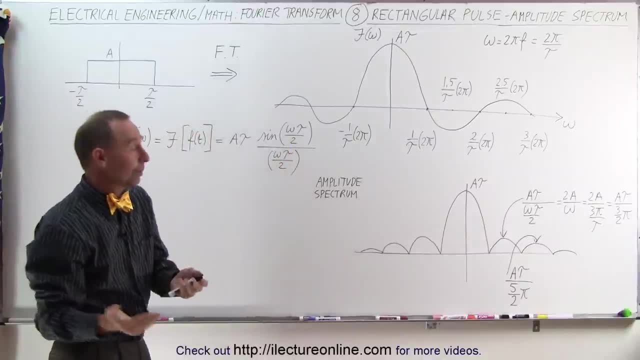 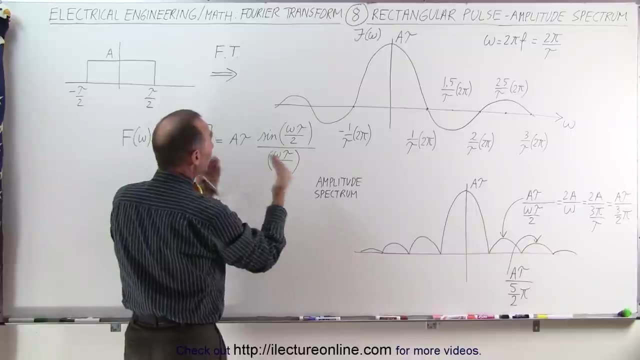 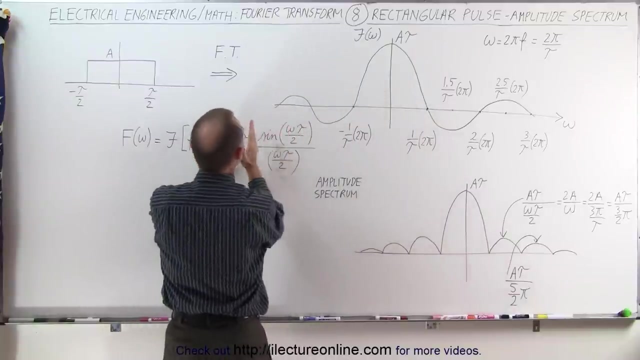 When the angle approaches 0, that ratio is always equal to 1.. By definition, in the limit as theta approaches 0, the sine of theta divided by theta equals 1. And therefore, when omega here is 0, you can then say that the amplitude is simply 1 times this. 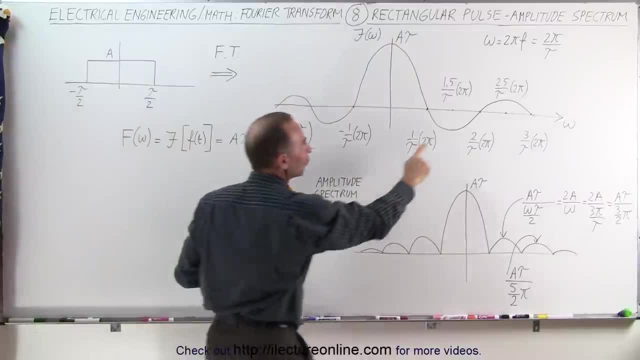 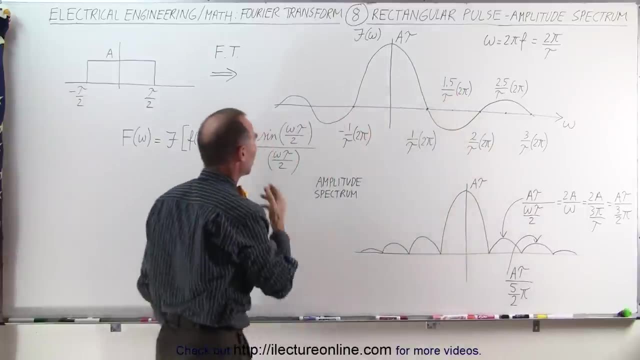 And therefore we get A times tau. But what about the amplitude, for example over here? Well, there omega is 1.5 times 2 pi over tau. So let's plug that in here and see what we get. 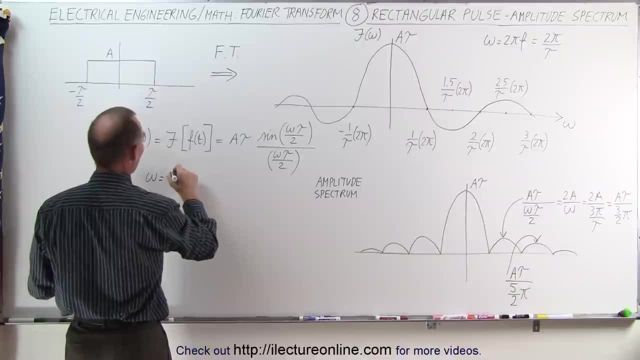 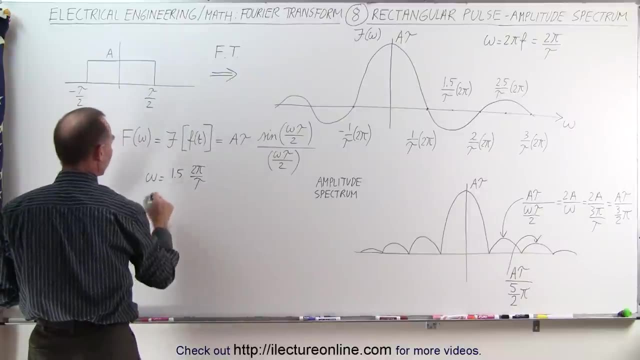 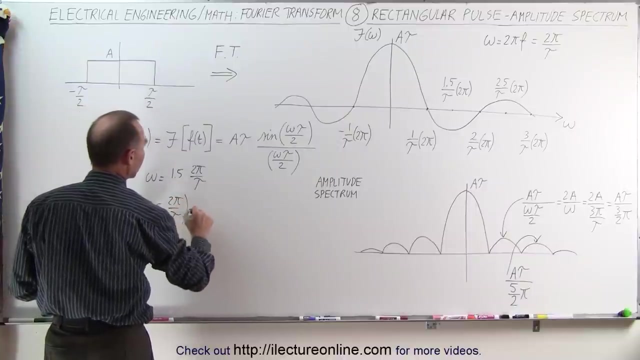 If omega is equal to 1.5 times 2 pi over tau, then what does this equal to? So then we can say that the function when omega is equal to 1.5 times 2 pi over tau is equal to A times tau times the sine of. 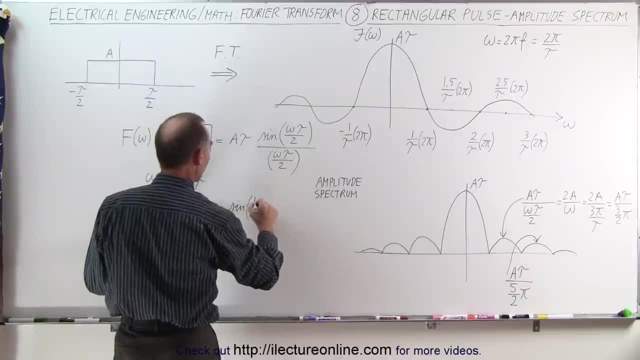 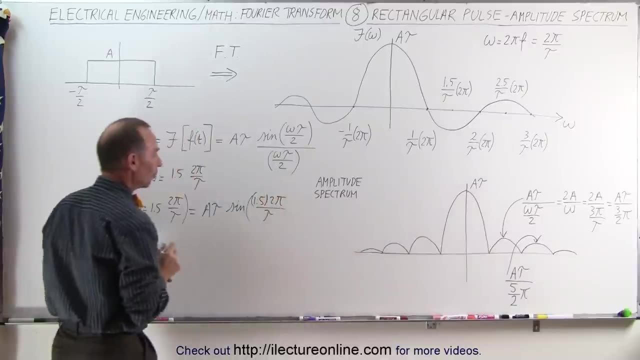 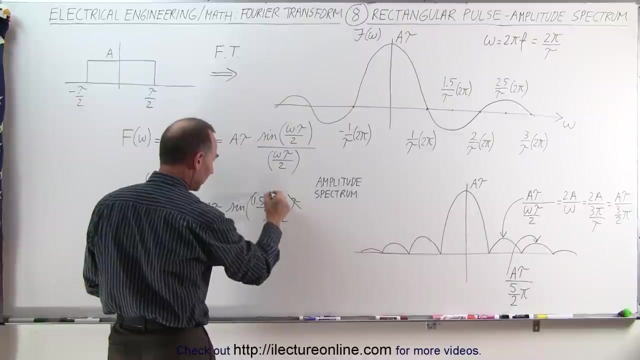 And so we plug in for omega 1.5 times 2 pi over tau, so 1.5, I'll put parentheses around it so it's clear- times tau divided by 2.. Notice that this cancels out, and this cancels out. 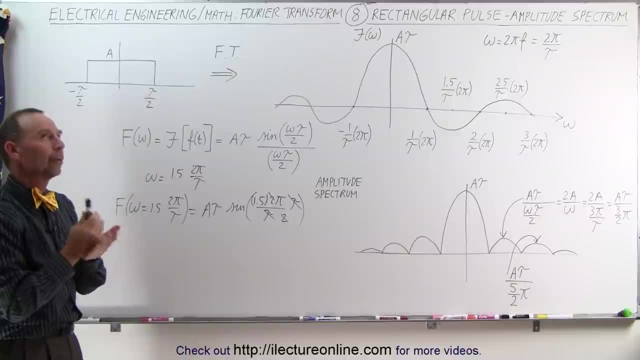 and we end up with 1.5 times pi. Well, 1.5 times pi, that's 270 degrees, And at 270 degrees the sine of that is 1.5 times pi. That is equal to negative 1.. 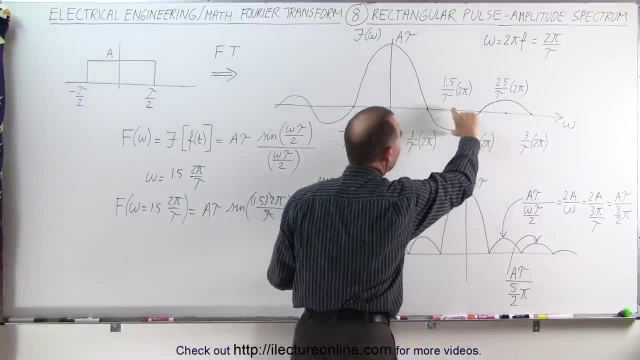 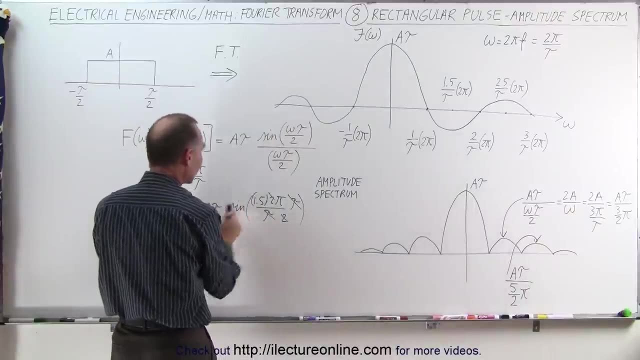 And so that's why you can see here at 270 degrees we end up with a negative amplitude. Then we have to divide that amplitude, so it would be negative 1 times this divided by this quantity. So when we calculate this, 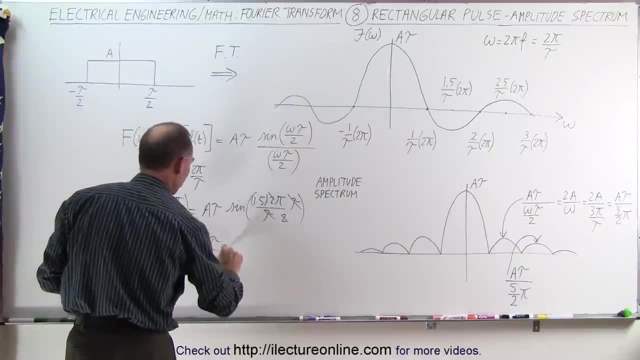 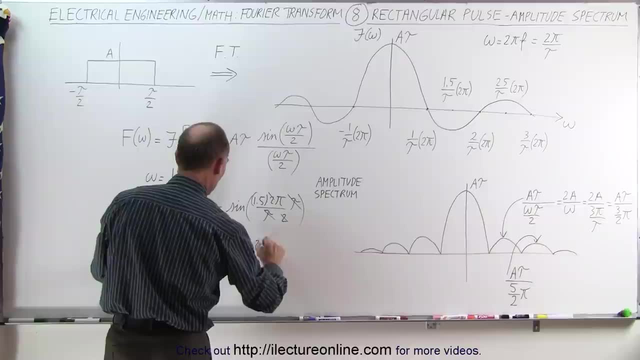 we can then say that omega tau over 2, when omega is equal to this right here, then we get 1.5 times 2 pi divided by tau times tau over 2, so the taus cancel out, the twos cancel out. 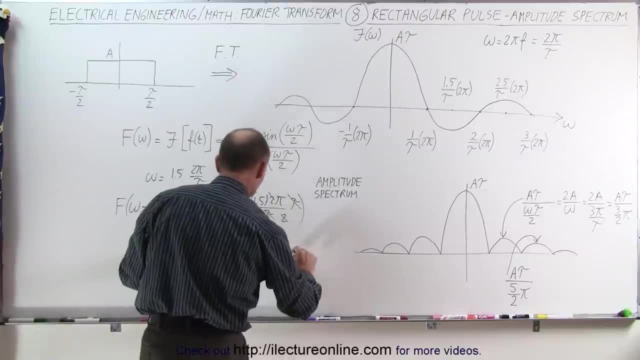 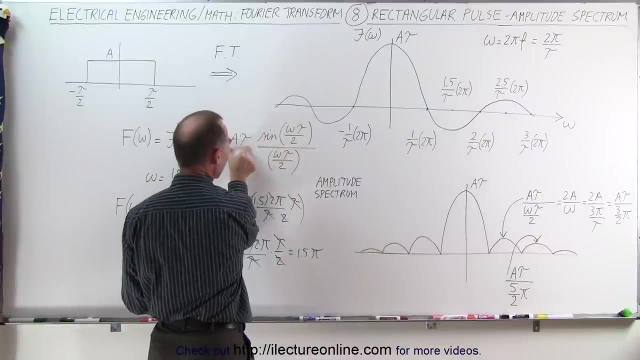 and we end up with 1.5 times pi. So this becomes 1.5 times pi and that goes in the denominator. so we end up with this magnitude times the negative 1, divided by 1.5 times pi. 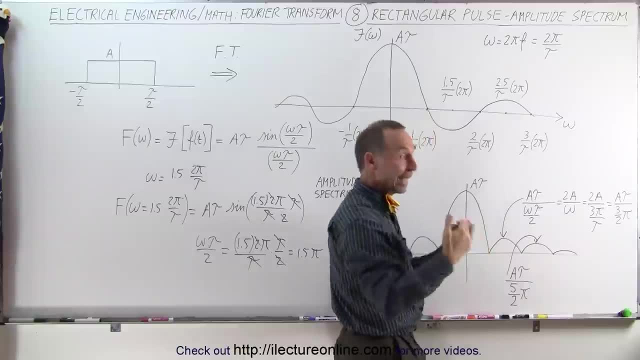 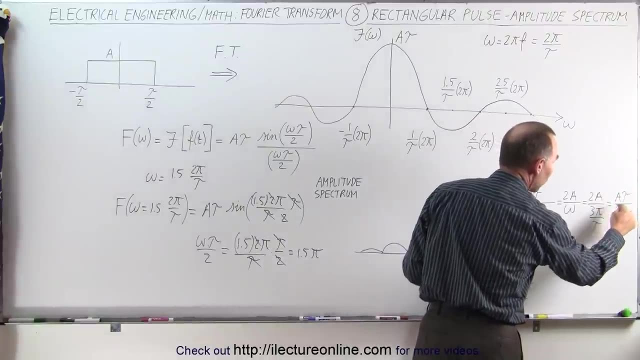 So therefore, the amplitude here we get rid of the negative, we end up with a tau divided by this. when we plug in the correct values, we get a tau divided by 1.5 times pi, and that will be the amplitude here. 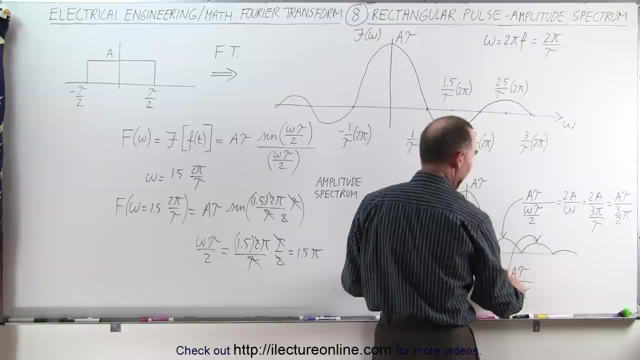 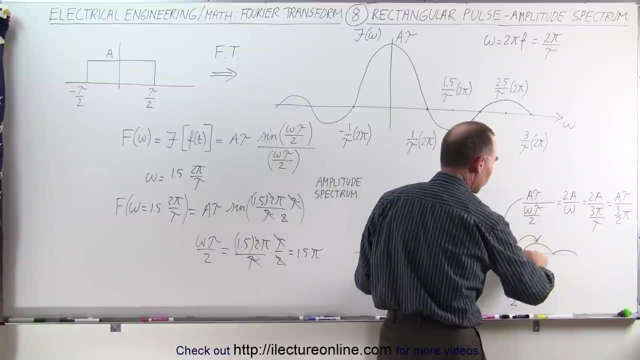 The amplitude for the next one here will be at times 5 over 2 pi, and the next one will be a tau divided by 7 over 2 pi, and so forth. so you can see that the amplitude keeps diminishing. 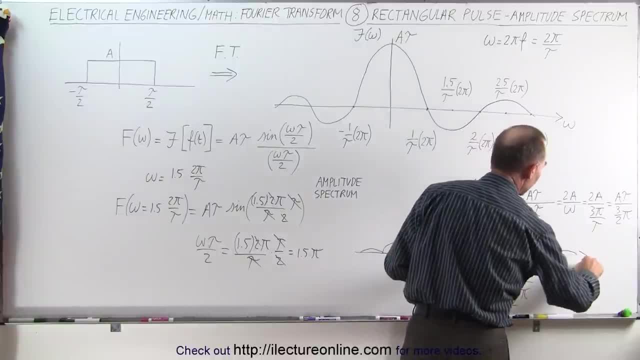 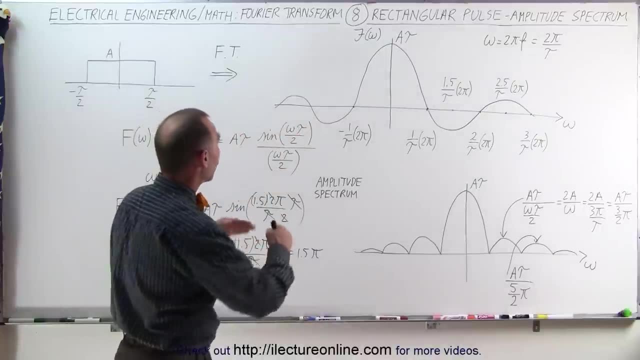 as you go farther and farther out in the frequency domain or on the frequency axis, I should say Alright, so hopefully that will give us a better picture of what this equation actually means. So this is the function. this is the Fourier transform of a single pulse. 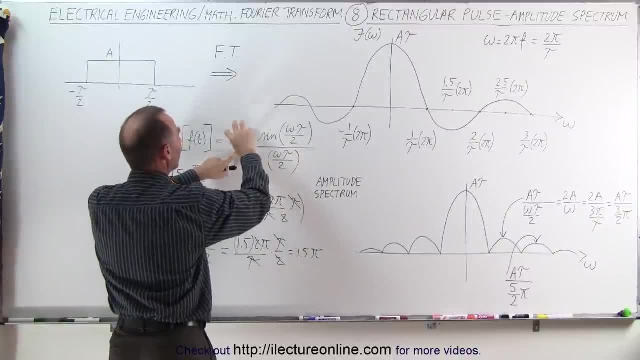 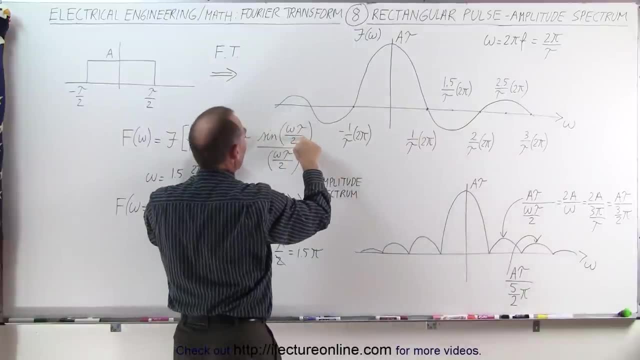 it is written in this format right here: it gives you this initial amplitude at the center and then, as you continue on, you can see you end up with a function that is the sine of omega tau over 2, divided by omega tau over 2,. 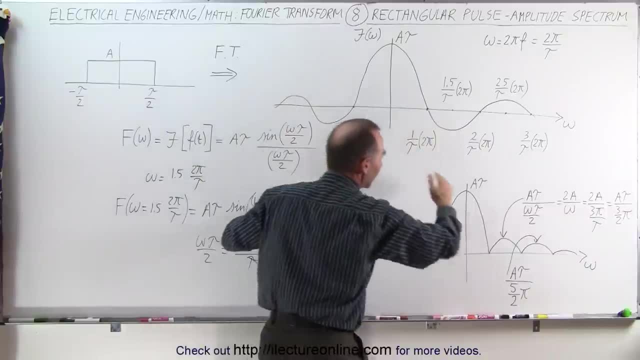 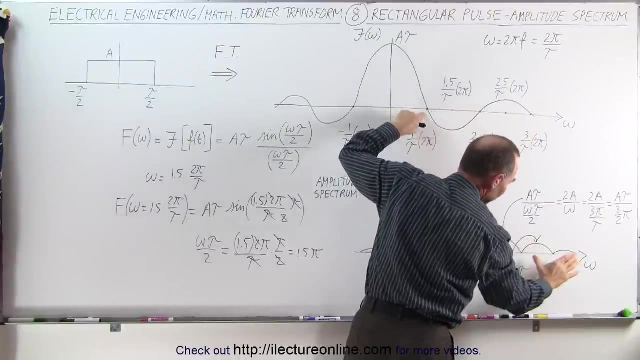 as omega gets bigger and bigger and bigger, you can see that the amplitude diminishes. if you then only take the positive of each of these lumps or each of these humps, you can see that this will be the magnitude of your Fourier transform. 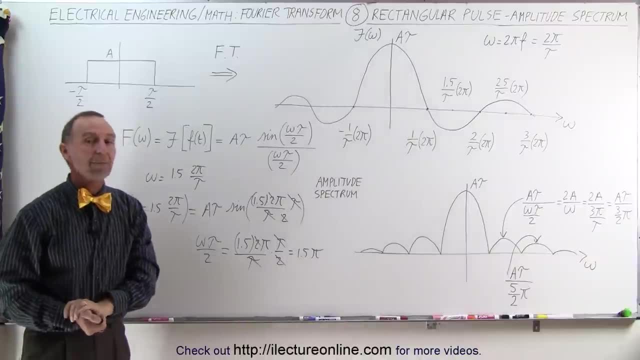 of this particular pulse, and that's what's called the amplitude spectrum, and that's how it's done. 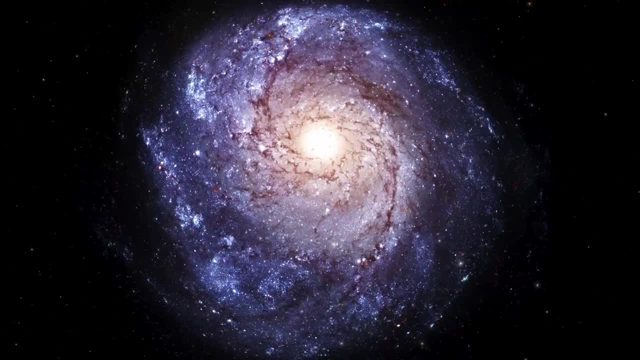 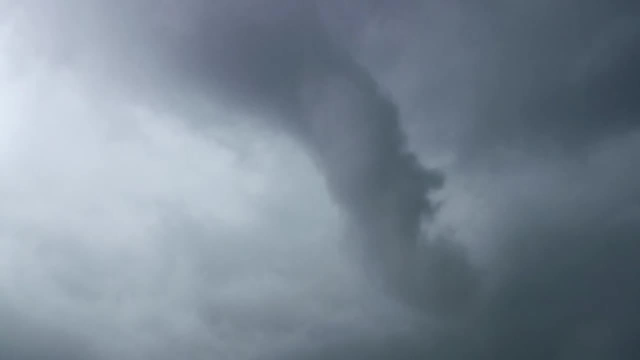 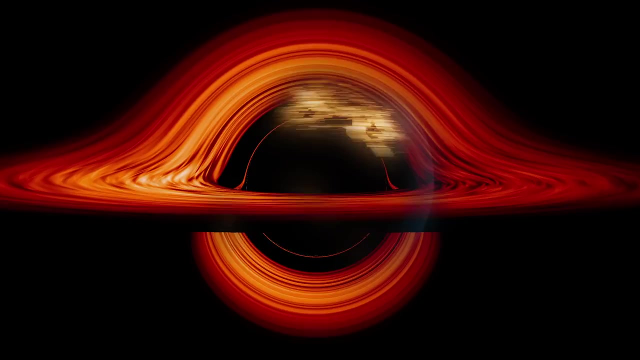 This is a video about one of the most important yet least understood concepts in all of physics. It governs everything from molecular collisions to humongous storms, from the beginning of the universe, through its entire evolution to its inevitable end. It may, in fact, determine the